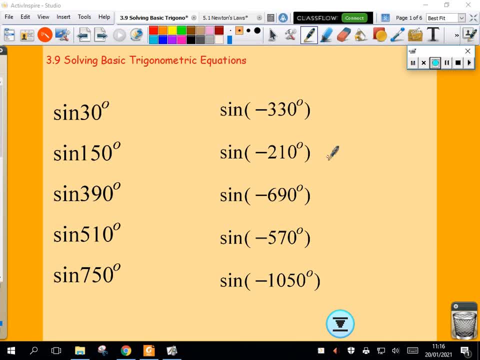 Okay, in this class I'm going to look at solving basic trigonometric equations. Just before I do, you know, if you pause your video there and just find, with your calculator, the sine of all these angles, of course, you shouldn't really need your calculator. 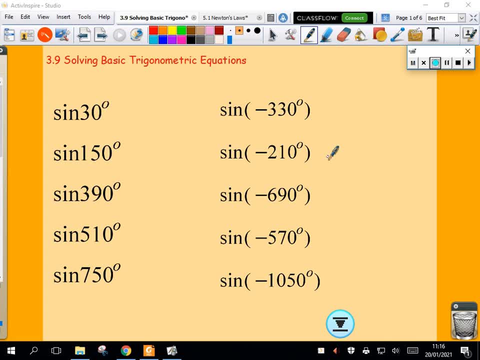 But if you do, type them into your calculator, make sure you're in degree mode, what you'll find is that every single one of these angles, every single angle, the sine is equal to a half. Every single one. All the way down, every single one is equal to a half. 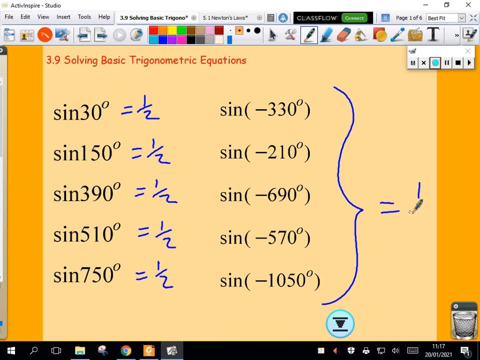 But again, all these in, every single one of those is equal to a half. And I could keep going on, you know, forever and ever. 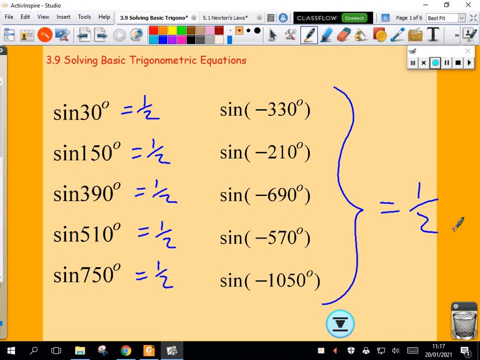 The point is that the sine of infinitely many different angles has a value of a half. 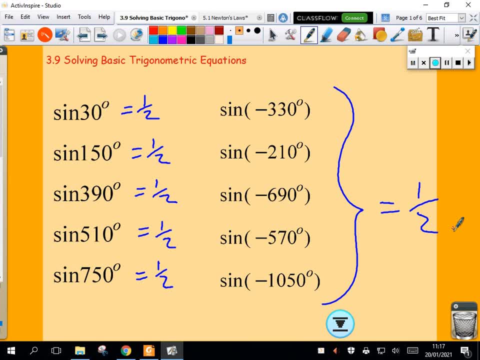 Because of how sine is defined. Remember, sine is defined as y over or. In the coordinate plane, the sine function is defined as y over or. 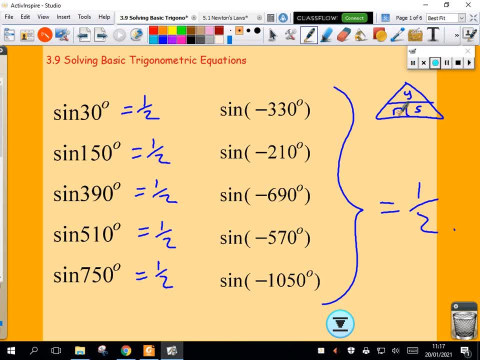 So anywhere where the y coordinate divided by or is equal to half, the sine of that angle will equal to a half. So I take anywhere, for example, two units away from the origin, where the y coordinate is one, that's two, that's one. The sine of that angle is going to be one half. But, you know, there's infinitely many angles that are coterminal with that. 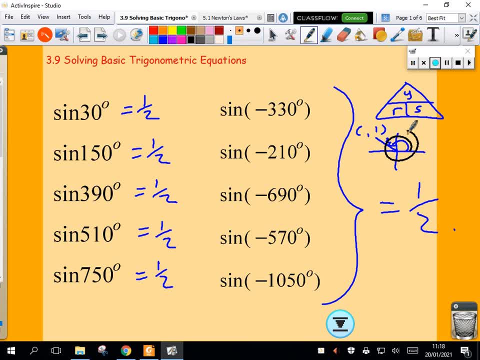 So suppose I went around, all the way around to 360 and then back to here and back there. There's another angle that has a sine equal to a half. Okay. 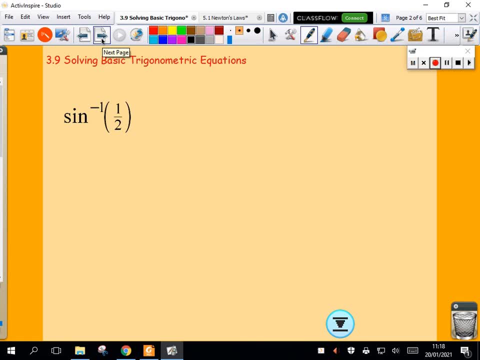 Now type your sine inverse function into your calculator, sine inverse of one half. And it will tell you that your answer is 30. It doesn't say. That there's infinitely many answers because they're not. The sine inverse of one half is 30 because of how we restrict the domain and the range for the sine function. 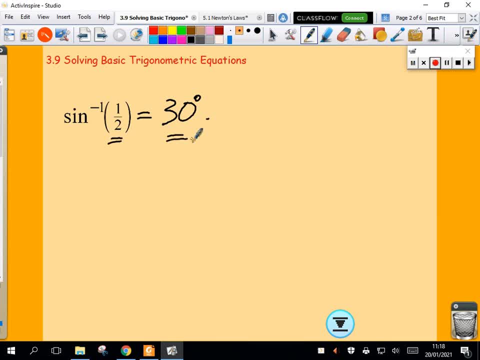 It's only a function if when I plug in one value, I can get one value out. 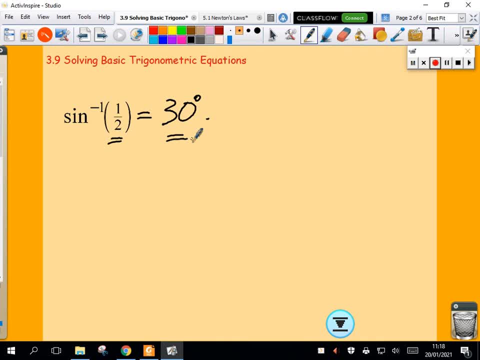 So what we do is we restrict the domain and the range. The domain is the numbers I'm allowed to get out. 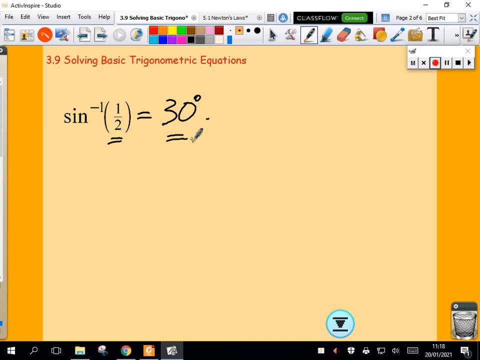 And the range is the numbers I'm allowed to. So the domain is the numbers I'm allowed to put into the function. 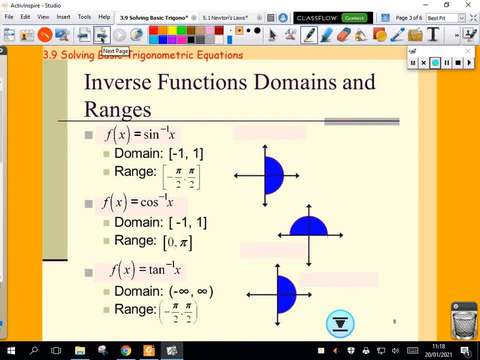 The range is the numbers I'm allowed to put out. So for the sine. 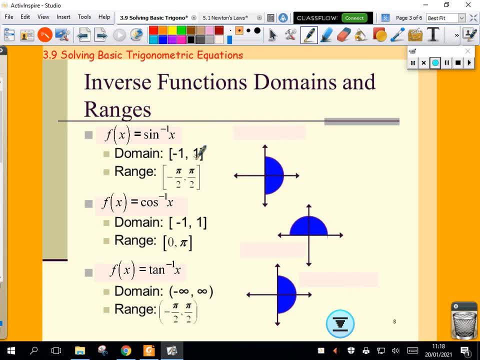 Inverse function, any number from negative one to one can go into the sine inverse function. So if you type into your calculator sine inverse of two, your calculator will tell you you've made an error because you're not allowed to put two into your domain. It can't go into the sine function. 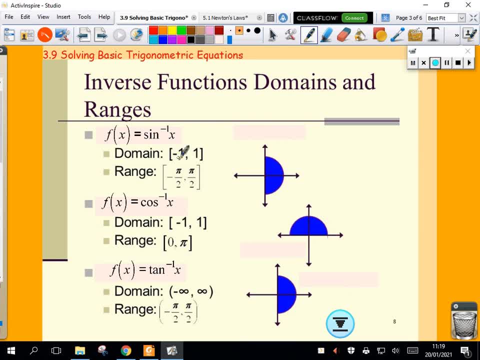 Only numbers from negative one to one. The square brackets mean negative one is included and one is included. And your range of the numbers you will get out. 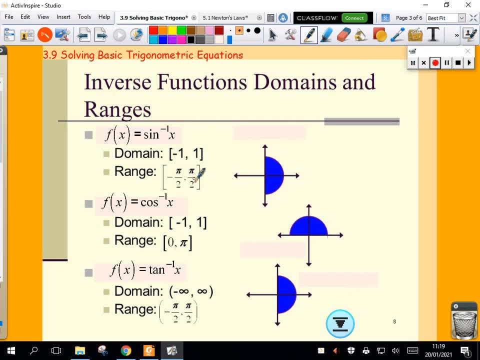 The range from negative pi over two. Radiance to pi over two. Radiance. 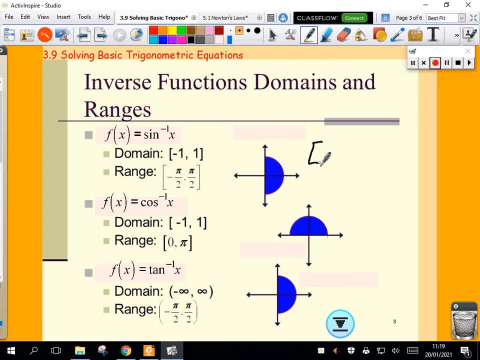 If I was to put that in degrees, negative pi over two will be negative 90 degrees to 90 degrees. So any time you type sine inverse of a number in, the number has to be between negative one and one. 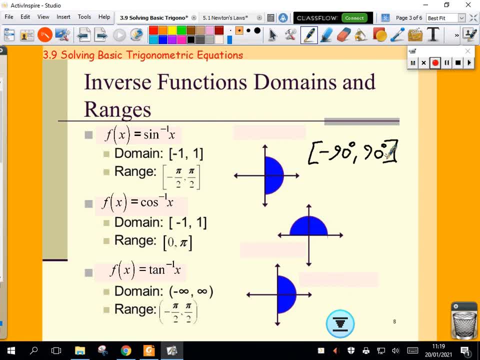 And the output you will get out will always be between negative 90 and 90. Or negative pi over two and pi over two. 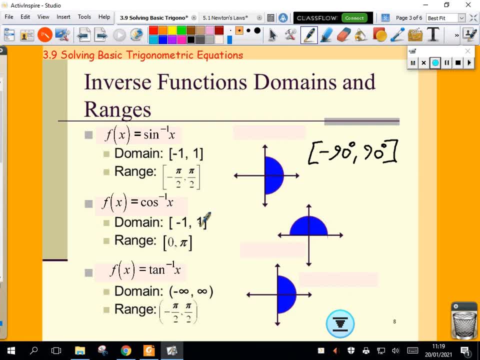 For the cosine function, the domain again is negative one to one. So if you try to type in cosine inverse. Five. Your calculator will tell you that's an error because it's not between negative one and one. Square bracket means negative one and one are included in this domain. And then the range, cosine inverse of any number you put in, will always be between zero and pi. In degrees, that will be between zero and 180 degrees. Remember, pi radians is equal to 180 degrees. 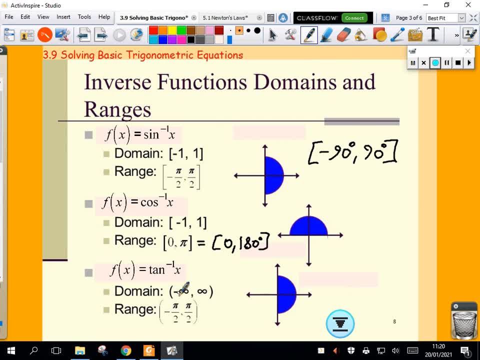 For the tan function, the domain is all the real numbers. You can plug any real number in here. Going from negative infinity as low as you like up to positive infinity as high as you like. Round brackets here because they're not actually included real numbers. Infinity isn't an actual number. Your range will be all the numbers from negative pi over two to pi over two. Which will be negative 90 degrees to positive 90 degrees. Notice the round brackets here because 90 and negative 90 are not included in this range. All the numbers between negative 90 and 90 can come out of the tan inverse function. 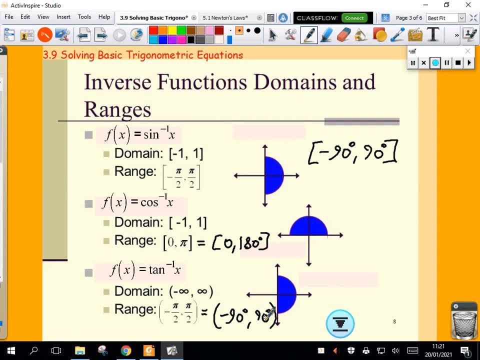 But 90 and negative 90 cannot. So round brackets say they're not included. Square brackets say they are included. And these are well worth remembering. The domain and the range. The domain is the numbers I'm allowed to put in. The range is the numbers that I can possibly get out. So you will never get, say, cosine inverse of some number. It will never, ever give you a hundred percent. Okay. 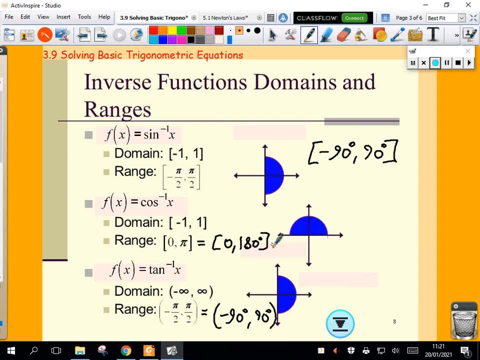 It's always between zero and 181. It's always between zero and 180. Okay. So we'll come back to it in a minute. 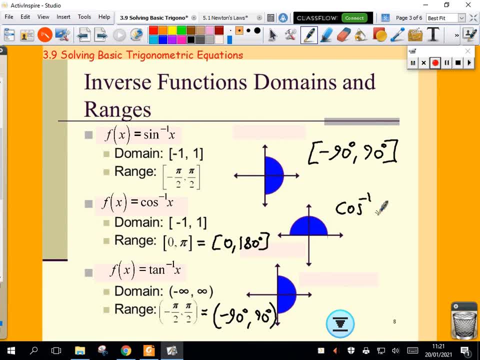 So if I was to ask what's cosine inverse of root three over two. Even though there are infinitely many angles whose cosine is root three over two. Cosine inverse of root three over two. Has to be between zero and 180. 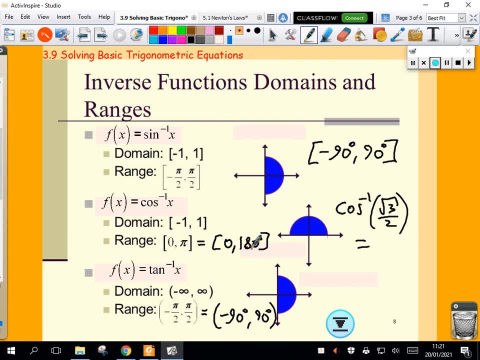 And the only angle between zero and 180 where the cosine is root three over two. Notice positive will be in the first quadrant. The only angle that that can be is 60 degrees. However, there are infinitely many angles whose cosine is 60 degrees. Infinitely many angles whose cosine is root three over two. For example, 60 degrees. 420 degrees. Okay. 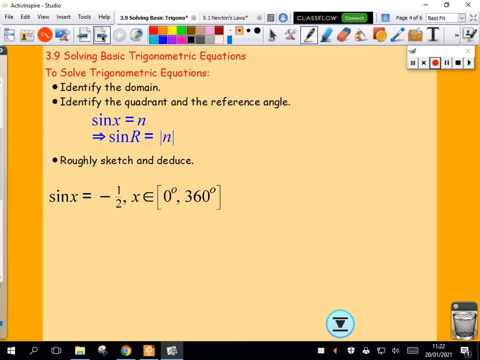 So let's look at a basic trigonometric equation. 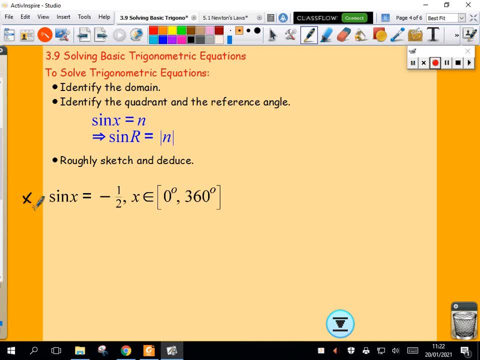 Here I have the question that says sine of x equals negative one half. We want to solve this thing. And x has to be between zero and 360 degrees. So solve this thing. Solve this equation is what we're being asked. 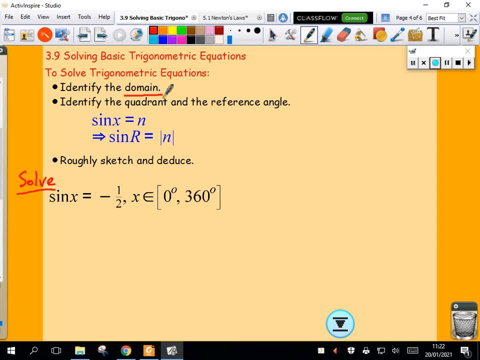 So a couple of things to understand. The first thing we always want to do is identify the domain. Okay. So the domain. 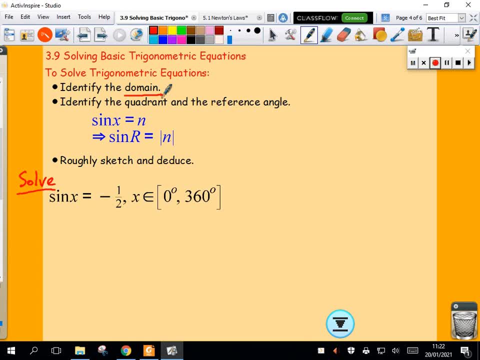 What is the domain? Well, there's a restricted domain. 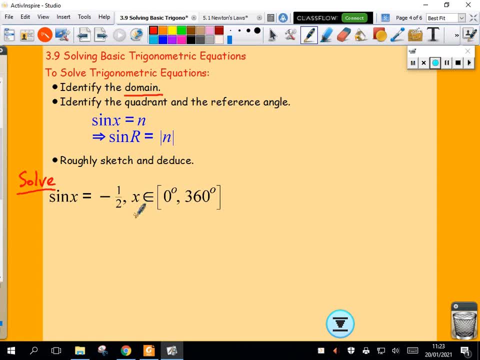 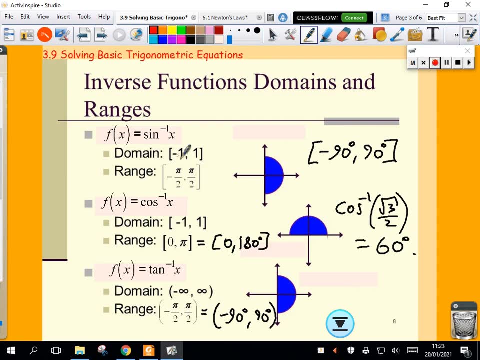 Generally with the sine function you can plug any number into it. You can find the sine of any number. The sine inverse function remember the domain can only be between negative one and one. 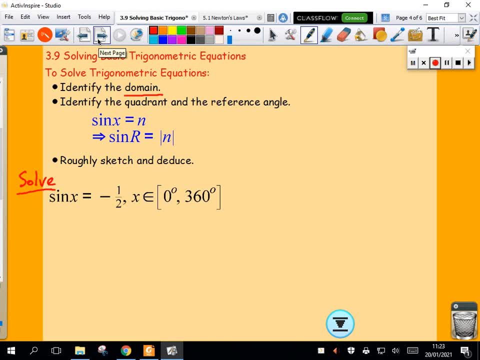 But for the sine function any number can go into it. However, they're giving me a restricted domain. They're telling me x has to be between zero and 360 degrees. So sine of x is negative one half. Remember that's the y coordinate divided by r. 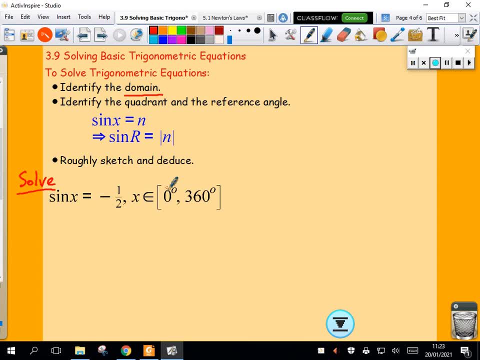 So the y coordinate would have to be negative one. And it would have to be two units from the origin. 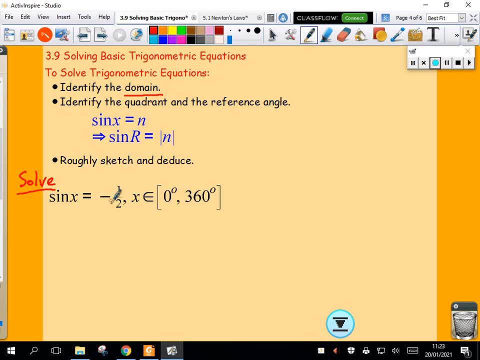 The first thing is to identify the domain. The domain here is this. It's given. It's between zero and 360 degrees. In general the domain for the sine function is all real numbers. However, in this question they're restricting it. 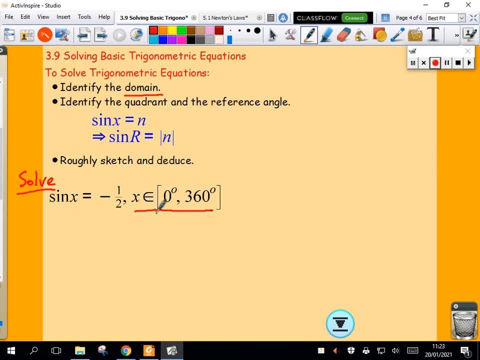 They're saying we want to find the values of x that are between zero and 360 degrees. 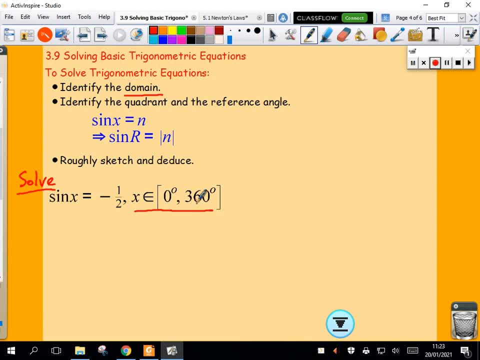 So find the values of x that are between zero and 360. That I can plug in here where the answer will be negative one half. So that's essentially what the question says. Find the values of x. 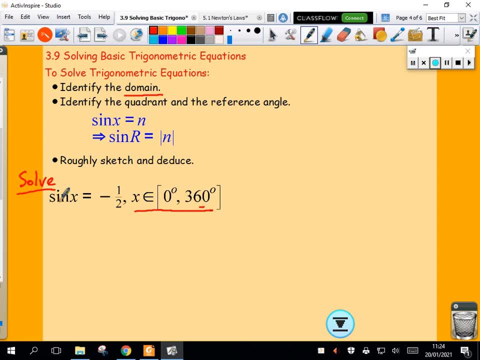 But they have to be between zero and 360. Where when I plug them into the sine function the outcome is negative one half. 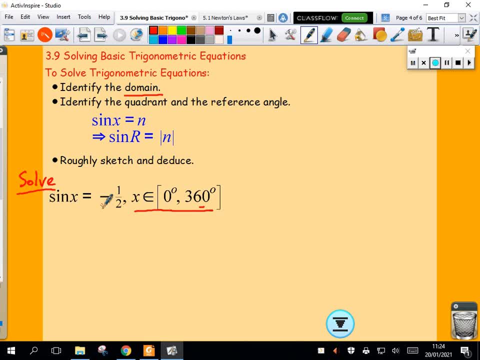 The second thing is to identify the quadrant and the reference angle. And we identify our quadrant. 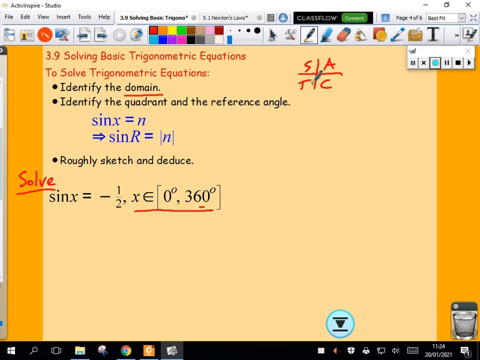 Using this kind of memory tool that we've spoken about. 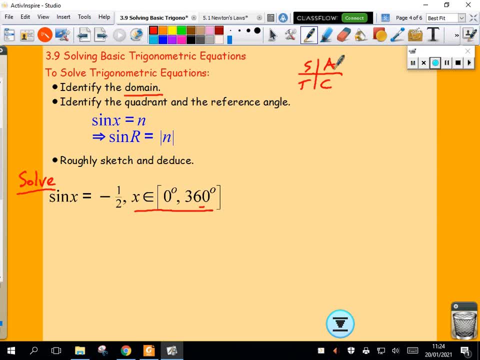 All trig functions have positive ratios in the first quadrant. Only sine and it's reciprocal in the second quadrant. Only tan and it's reciprocal in quadrant three. And only cosine and it's reciprocal have positive ratios in quadrant four. 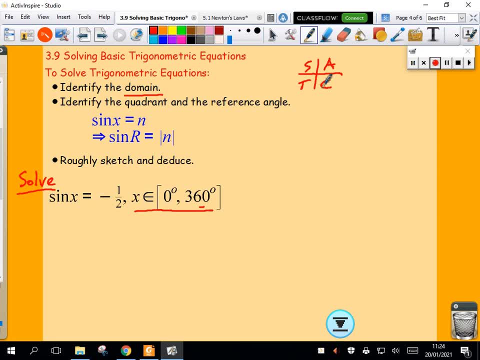 To identify the reference angle we'll remember if sine of x is some number. Then sine of the reference angle will be. The absolute value of that number. The reference angle is always an acute angle. 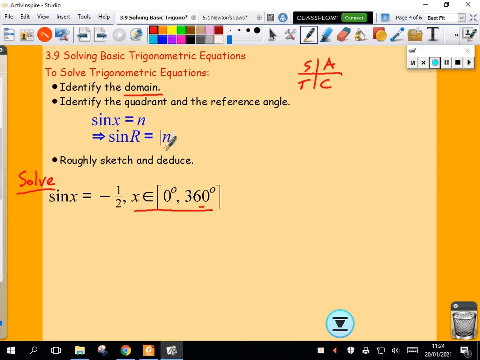 The sine of any acute angle is always a positive thing. Then we just roughly sketch and deduce our answer. Once we've done those first couple of things. It's really plain sailing. We just have to think logically. 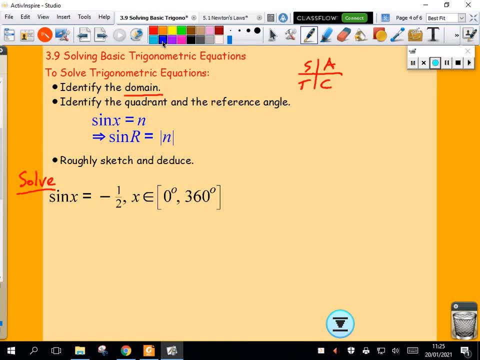 So we're going to try to solve this thing. The first thing is identify the domain. The domain is given. Let me read this. Let me write it out here. 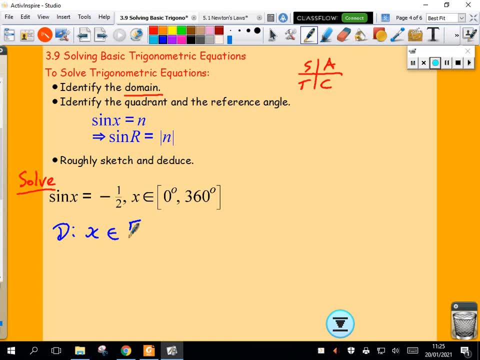 The domain is x belonging to the interval from zero degrees to 360 degrees. So any number between zero and 360 degrees could be the answer here. So we're going to narrow it down by identifying the quadrant. So sine of x is negative a half. 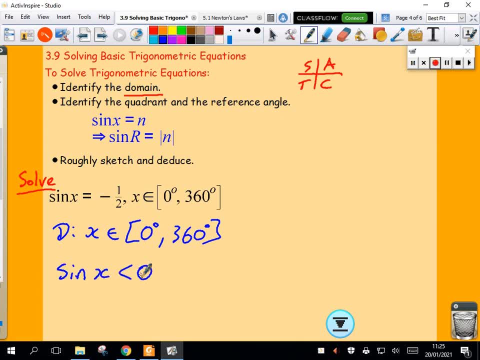 And we know that the sine of x is negative in quadrants. When we look up here. 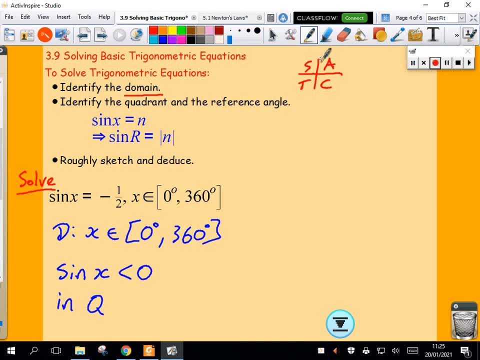 All functions are positive in the first one. 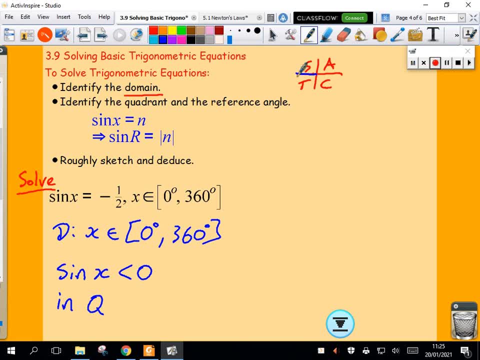 Sine is positive in the second one. So sine is negative in there because only tan is positive. 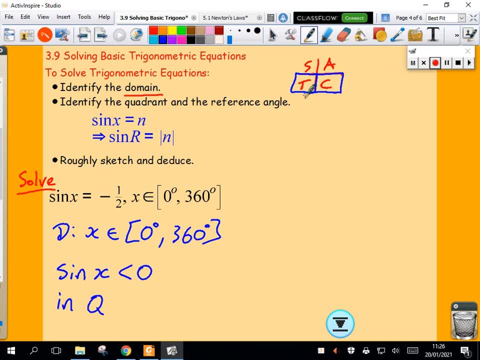 And sine is negative also in there. So sine is negative in quadrants three and four. 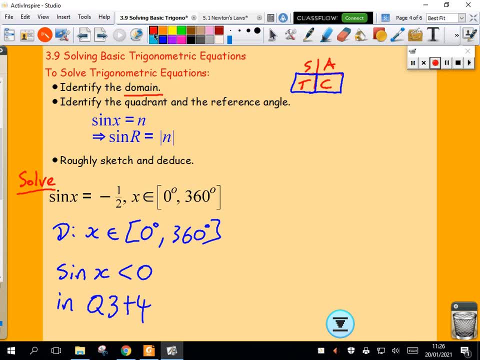 So I've identified the domain. I've identified the quadrant. And now I want to find the reference angle. 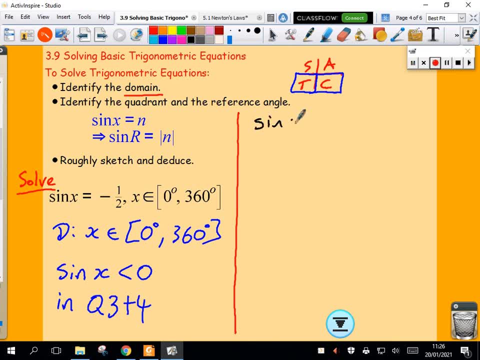 So sine of x is negative one half. Well that means sine of the reference angle is the absolute value of negative one half. It's positive one half. 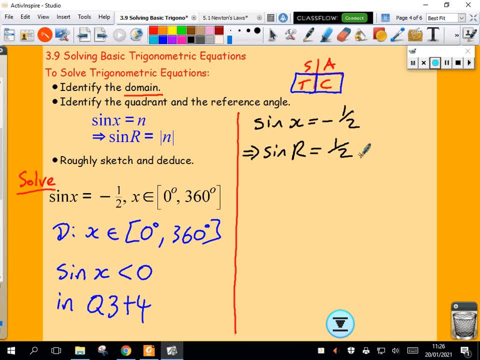 So sine of the reference angle is positive one half. 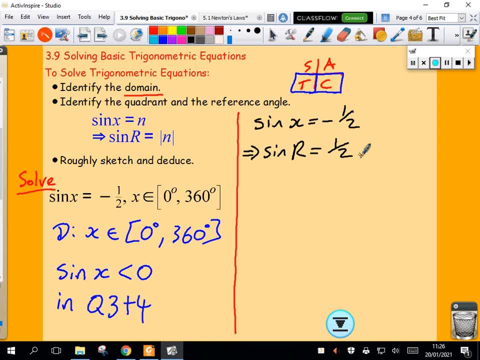 I want to identify the reference angle. The sine of what angle is positive one half. 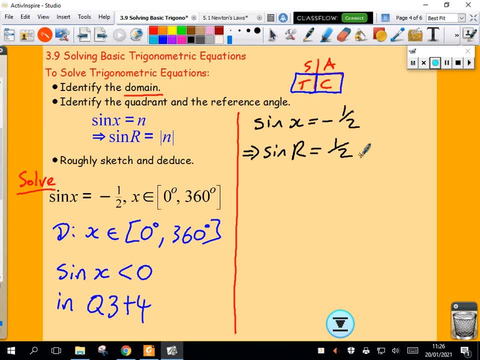 So to find the reference angle you probably know it already. If you know your special angles. 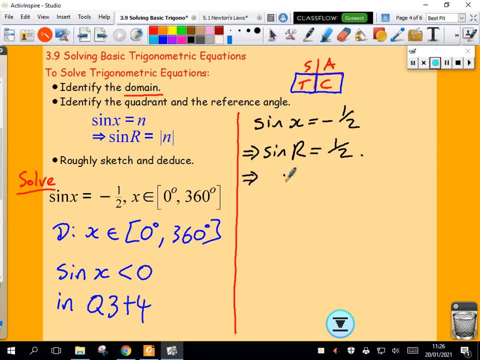 But if you don't and you have a calculator. You can just type in the reference angle will be sine inverse of one half. Okay. 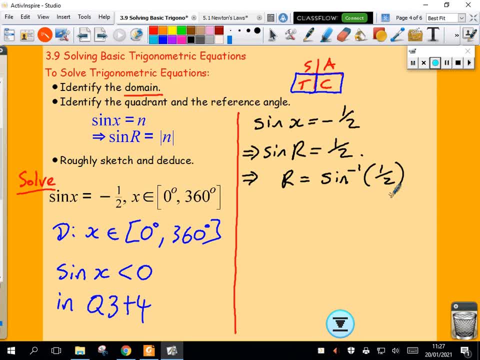 Sine inverse of one half. And you plug that into your calculator. 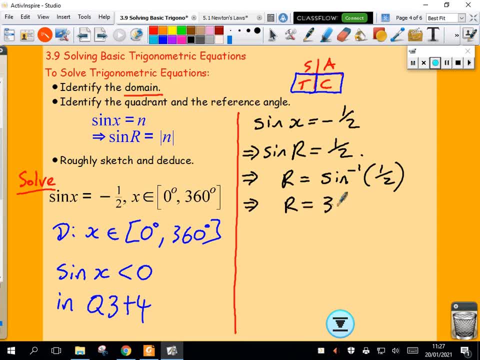 You'll find the reference angle is 30 degrees. 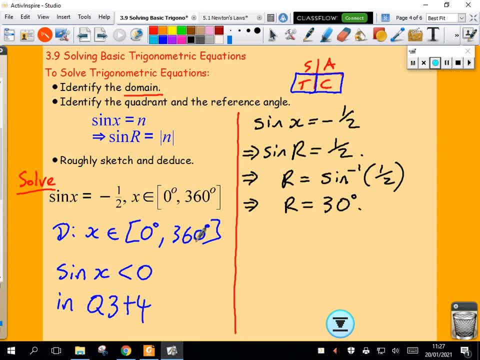 I should of course identify that the domain is given in degrees. So my answer has to be degrees. 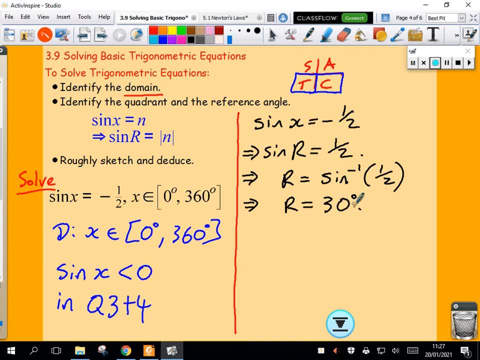 I'm dealing with radians here. So my reference angle is 30 degrees. Again going through my steps. 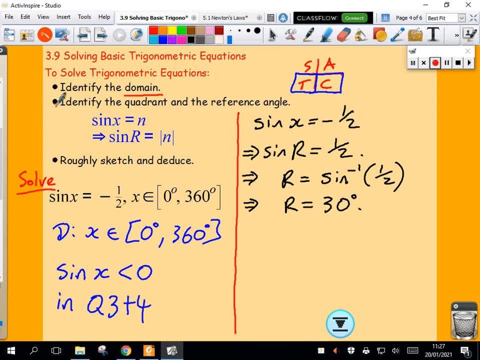 All the numbers from zero to 360. Identify the quadrant and the reference angle. We saw that sine was negative. Therefore in quadrant three and four. Sine of the x is negative one half. So sine of the reference angle is positive one half. Working that out we can figure out that the reference angle has to be 30 degrees. Now finally we're going to sketch and deduce an answer. 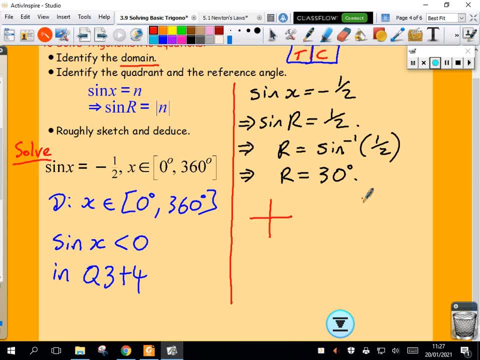 So we're going to draw. 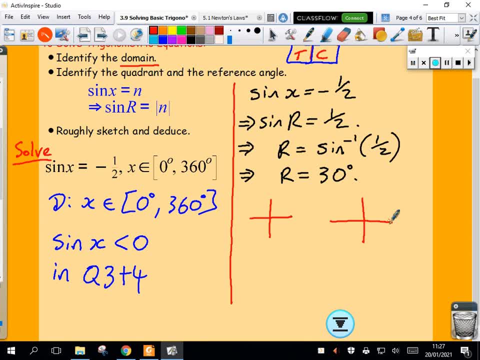 Remember we're dealing with quadrants three and four. 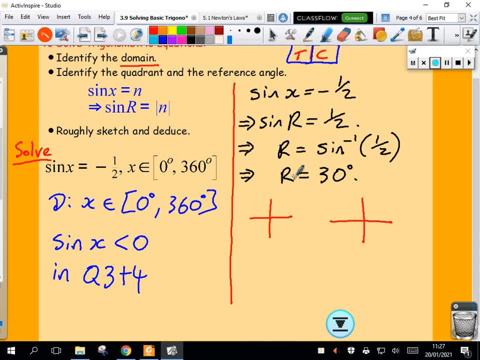 We're dealing with a reference angle of 30 degrees. So reference angle of 30 degrees. 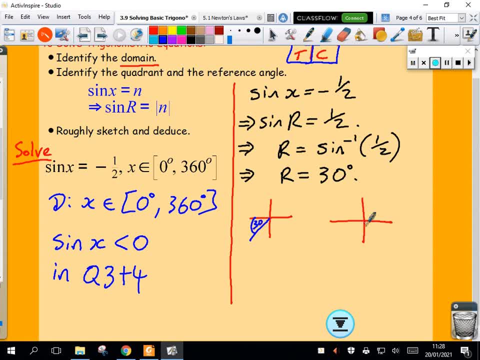 There's quadrant three. Quadrant four reference angle 30 degrees. 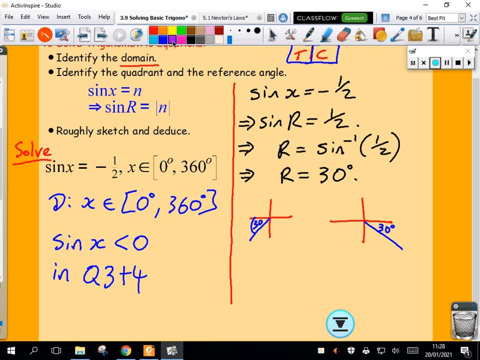 There we are. The angle x could be either this angle all the way around here. Or this angle all the way around here. So we just have to deduce what are those angles. 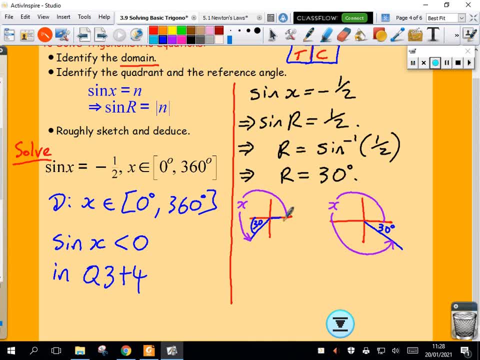 So remember there's zero degrees, 90 degrees, 180. And this is going to be 180 plus 30. So x in this case would be 180 degrees plus 30 degrees. 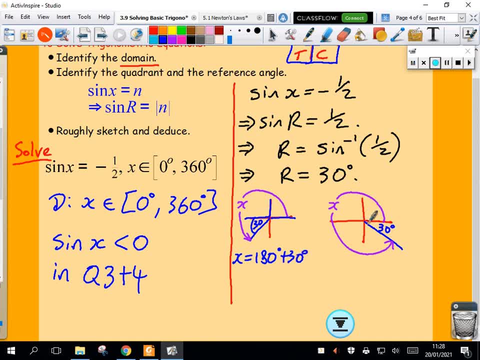 And over in the second case. We've got zero degrees, 90, 180, 270. Around here would be 360. But we're not going. We're going 30 degrees less than 360. So hopefully you can see that x in here would be 360 degrees minus 30 degrees. 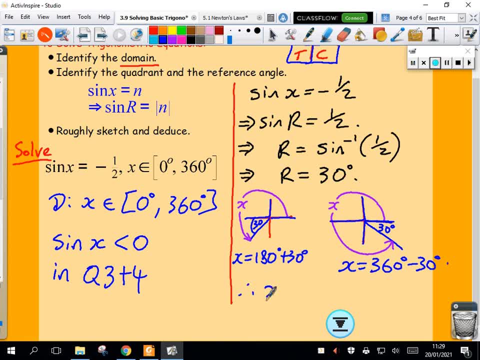 So therefore x can be one or two things. Okay. 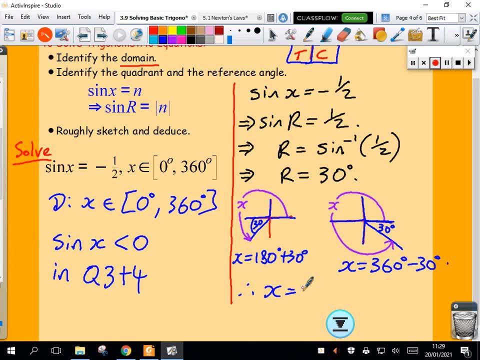 It's either. 210 degrees or 330 degrees. 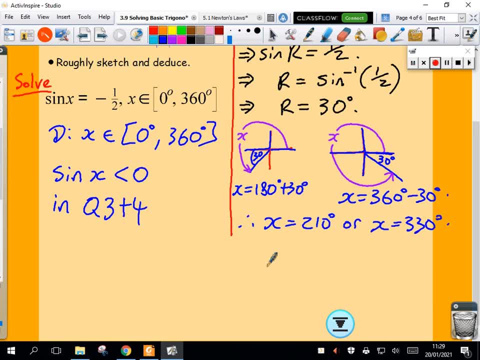 And they're the two angles. Sometimes you see that written in set notation. X belongs to the set. Set brackets here. Chain brackets important. Containing the elements. 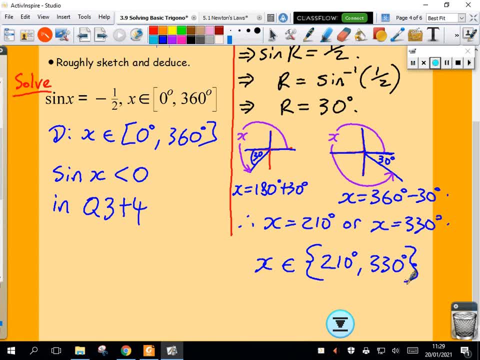 210 degrees or 330 degrees. So x could be one of those two things. 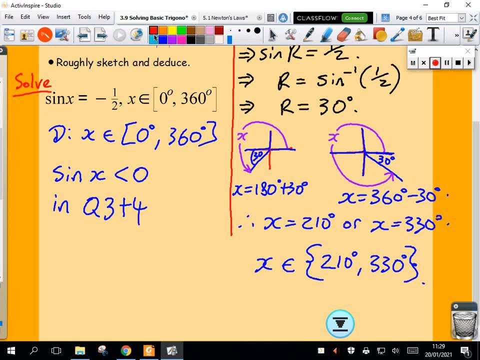 And again type those in. Check your answer. How do you check your answer? Well you first of all. Are those answers fitting into my domain? Yes. They're both between zero and 360. And check. 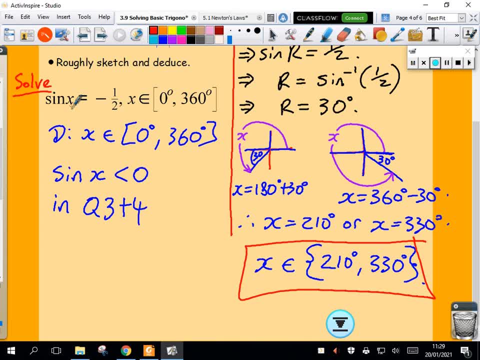 Is sine of the angle equal to negative one half? Okay. Really common error with this question is people just take it and write in sine inverse of negative one half. That is not giving me my answer. Because it's not giving me all my possible values between zero and 360. Note. Let me just type in. 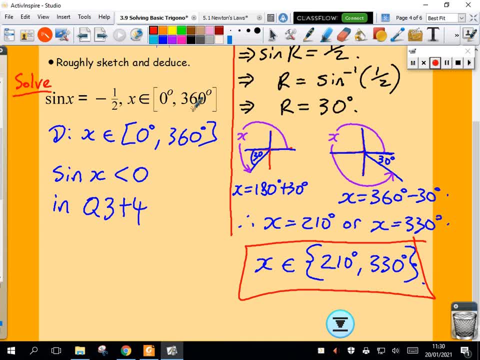 Sine inverse of negative one half into my calculator. 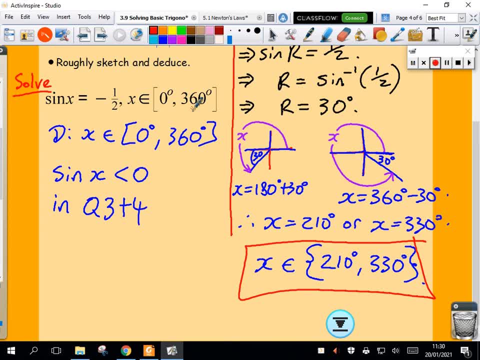 And your calculator tells you it's negative 30 degrees. Notice negative 30 degrees does not come up in here. Okay. What negative 30 degrees? Notice there's a negative 30 in there. That's that. 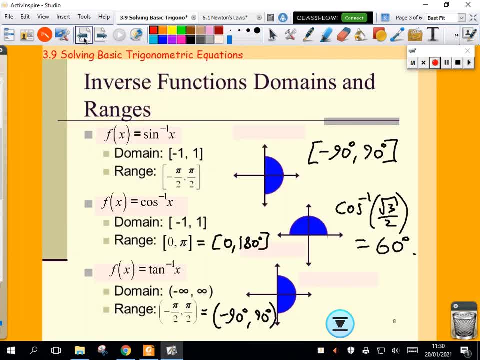 Why is my calculator telling me negative 30? Well your calculator will always tell you values between negative 90 and 90. Okay. 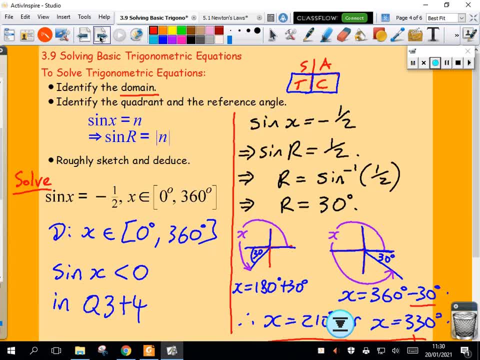 So your negative 30 fits in there nicely. However, it doesn't say find sine inverse of negative one half. It says if sine of some angle between zero and 360 degrees is negative one half. Then find that angle. Okay. And there are two of them. 210 or 330 degrees. So follow the steps. All of these can be solved in the same way. 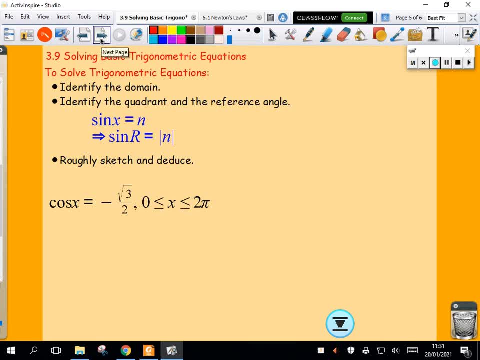 Let me look at another example here. So sine of x is negative root three over two. Here my domain says zero is less than or equal to x. Which is less than or equal to two pi. So I have to work this out in radian mode. Okay. So if you're using your calculator. Make sure the first thing you do is change your calculator to radian mode. 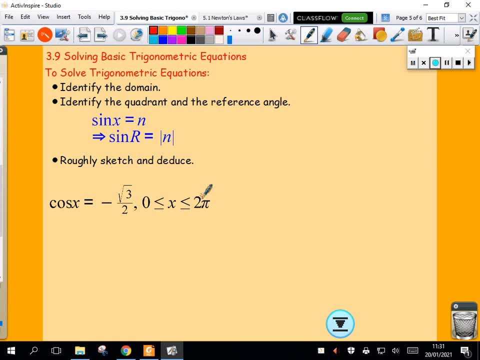 On my calculator I do that by hitting shift. Setup. Press number two for the angle unit. And then number two for radians. Okay. 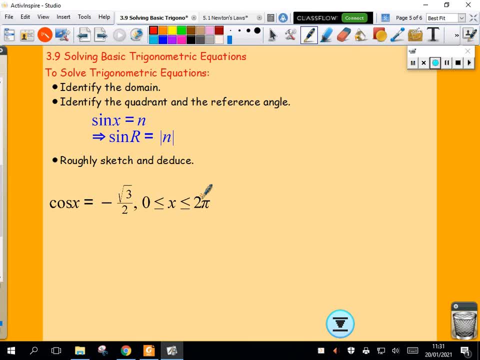 But you'll have to figure out your own calculator if you have a different one to mine. 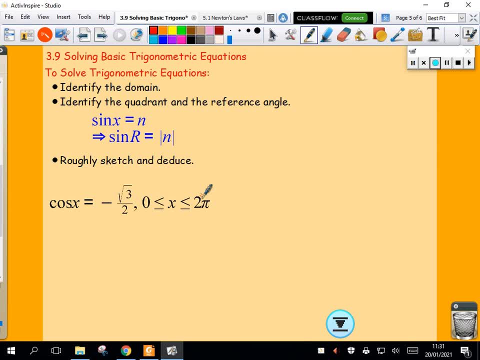 So cosine x equals negative root three over two. This is my domain. Step one identified the domain. 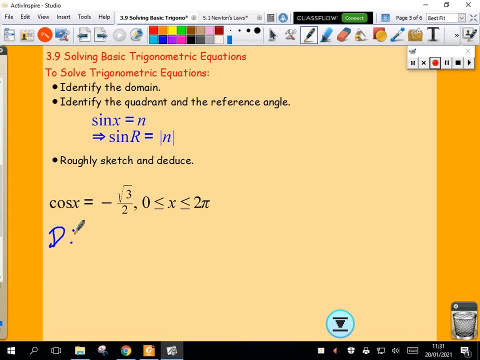 So the domain here is x has to belong to the interval starting at zero and finishing at two pi. Okay. Including. Notice square brackets here saying including zero and two pi. Because it's a less than or equal to sign. So zero is included. Two pi is included. That's my domain. If you prefer to use it. 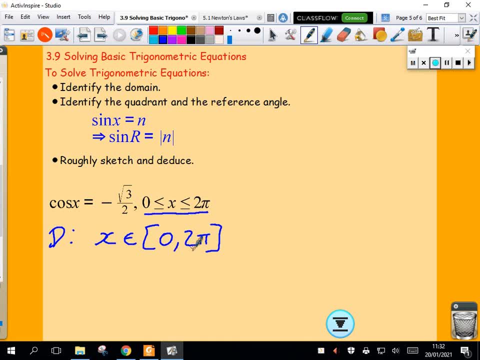 An inequality as opposed to interval notation. Feel free. 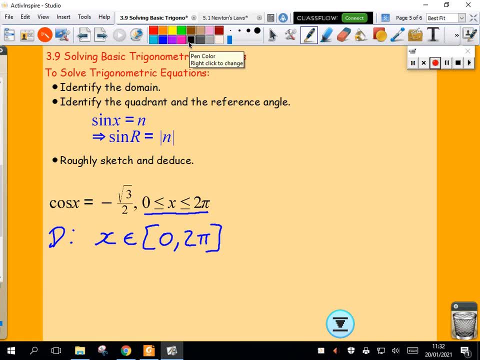 Whatever you prefer. So that's my first thing. I'm identifying the domain. 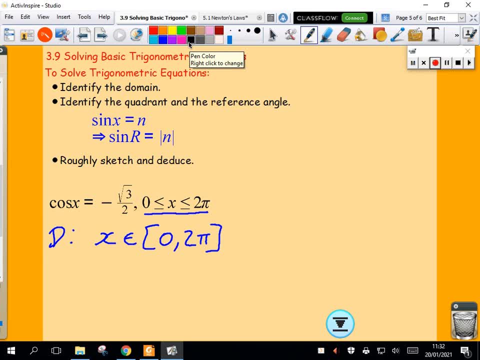 The second thing is to identify the quadrant and the reference angle. So cosine of x is negative root three over two. So I'm just going to say cosine of x is negative in quadrants. Again. 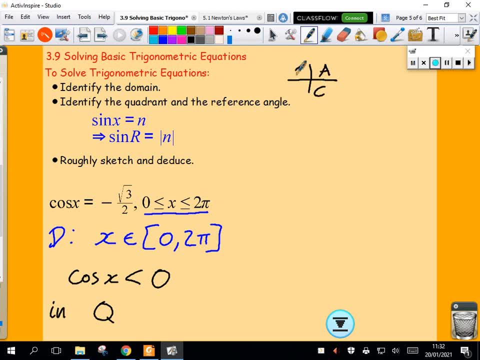 You can use your little memory tool. And you'll see that cosine is positive in quadrants one and four. 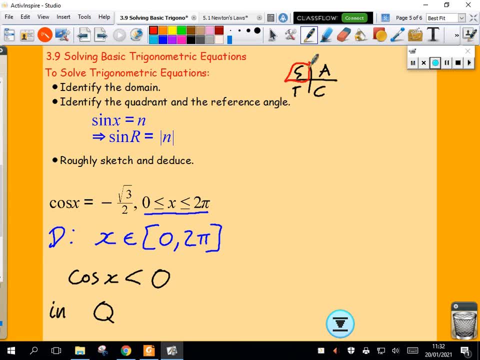 So cosine is negative in here in quadrant two and in here in quadrant three. So cosine is negative. That means we're dealing with quadrant two and three. 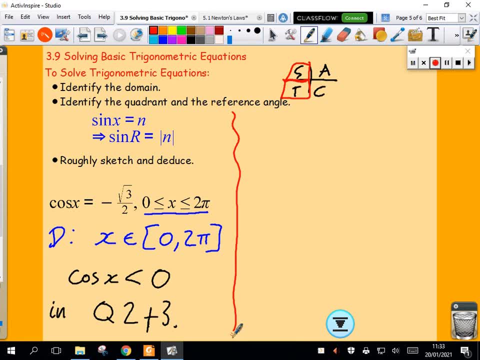 The next thing is to find the reference angle. And again to find the reference angle. We're going to say well cosine of x is given as being negative root three over two. Which means that cosine of the reference angle will be the absolute value of that positive root three over two. 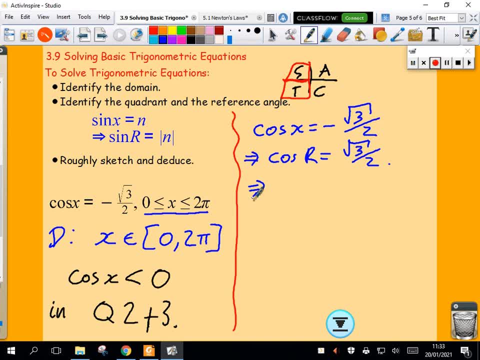 And you should really know what reference angle will give you root three over two. When you plug it into the cosine function. I know it already. I know it's thirty degrees. 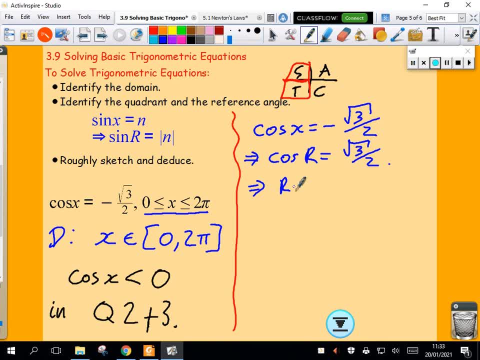 But if you don't. Type into your calculator. Cosine inverse of root three over two. 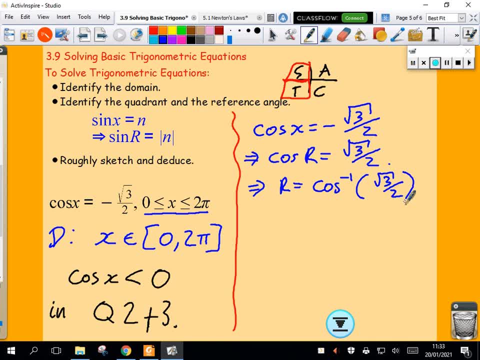 Cosine inverse of root three over two is thirty degrees. Or if we're in radian mode. 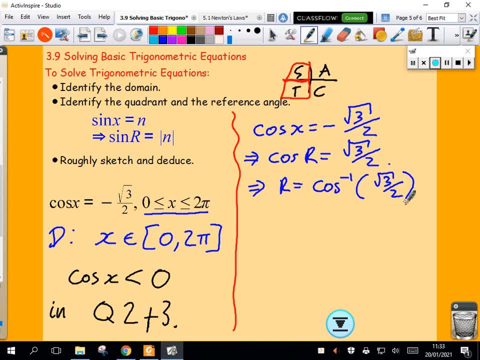 That's going to be pi over six. Okay. So depending. Again you can use both. 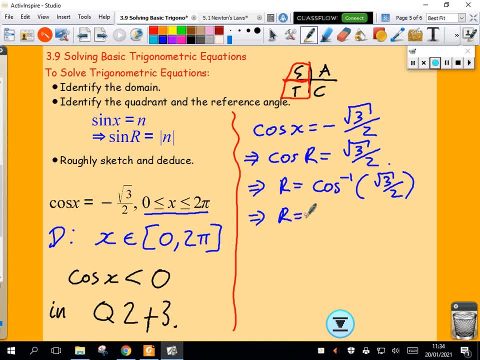 As long as you give your final answer in radians. Use degrees along the way. I'm going to use radians. But you could. You could say. 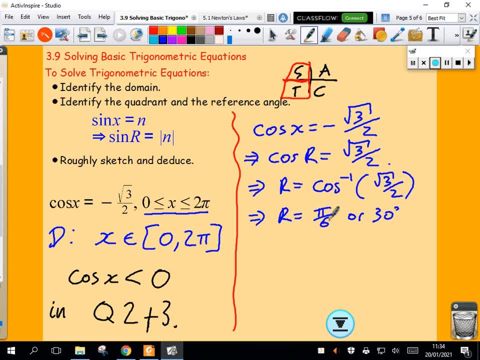 Thirty degrees at this stage. My final answer ultimately has to be in radians. 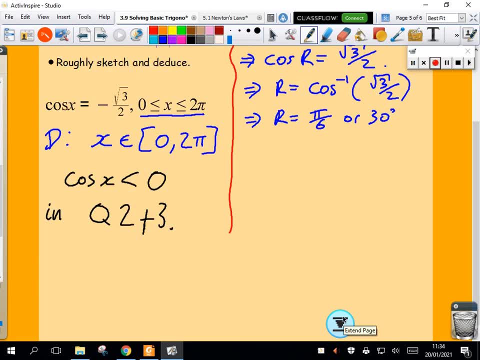 But if you prefer using degrees. You know. Feel free. At this stage. Using your reference angle. No problem. Okay. So now. I've found my reference angle is pi over six radians. Or thirty degrees. 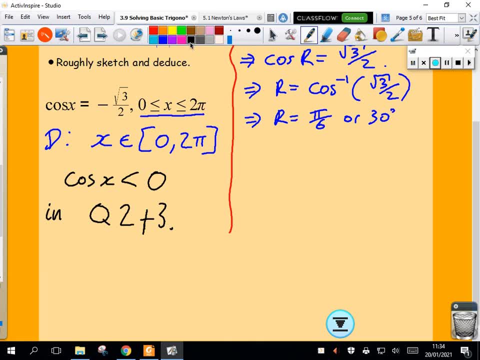 I know I'm in quadrant two and three. Now I'm going to sketch. 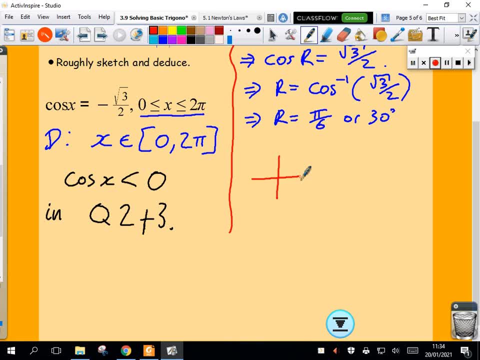 So sketch. And deduce. So sketch. Quadrants two. 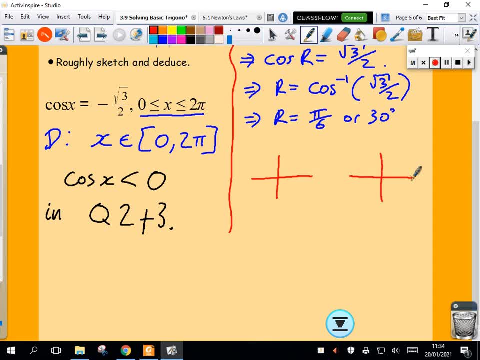 And three. So in quadrant two. 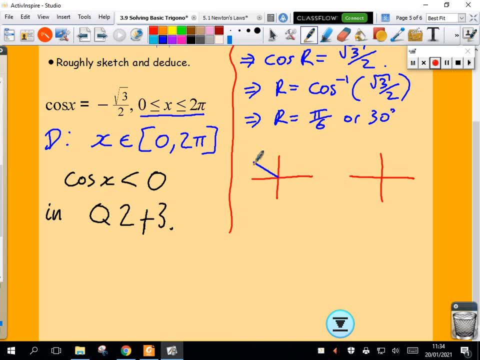 Reference angle of pi over six. Quadrant three. Reference angle pi over six. If you prefer to stay with degrees for the moment. And then convert into radians at the end. That's fine. I'm not going to do that. Remember. A straight angle. Around two one hundred and eighty degrees. That's zero radians. 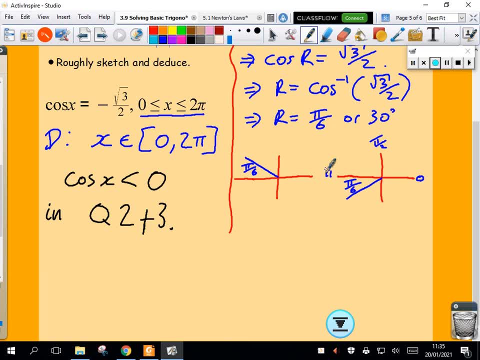 Pi over two radians. Pi radians. So this is. 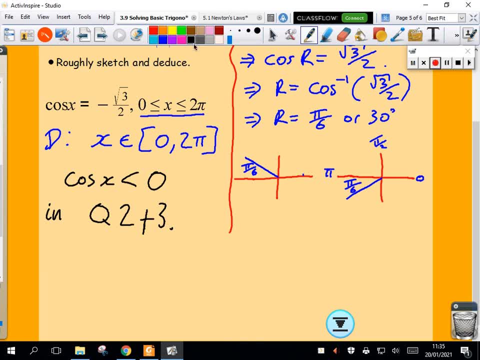 In this first one. The angle we're looking for here. X. 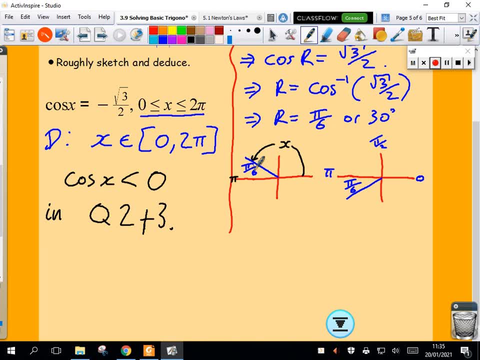 Well it's going to be. Pi radians. But subtract pi over six. So x would be. Pi radians. Subtract pi over six. In this. Quadrant in here. 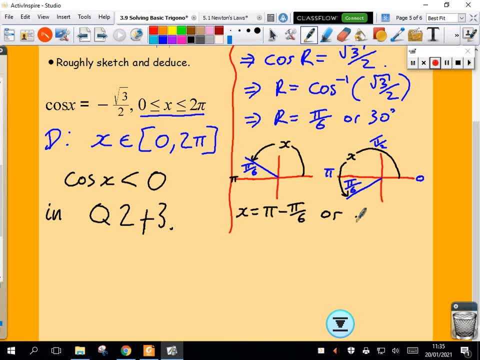 You know. X would be. Pi radians. Plus pi over six. So. X is going to equal to. Pi. Is just six pi over six. So six pi over six. 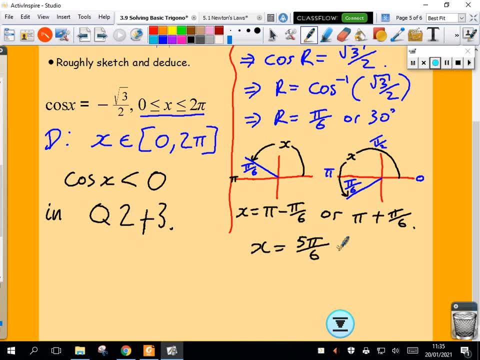 Minus one pi over six. That's five pi over six. Pi. Plus pi over six. Well that's six pi over six. Plus one pi over six. That's going to be seven pi over six. So there's my answer. It's one of those two things. 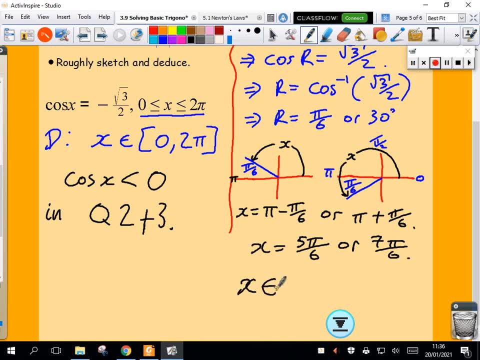 If you prefer set notation. Again you can write that. X. Belongs to the set containing. The elements five pi over six. And seven pi over six. So either of those. Answers is good. So you can write it like that. Or. Like that. Depending. 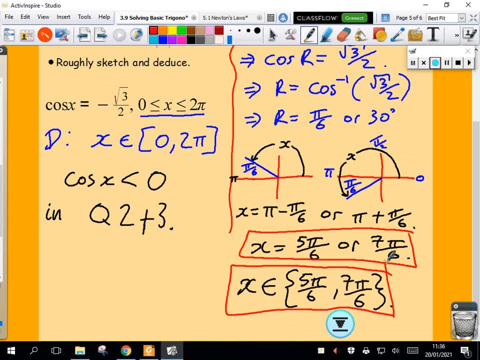 On personal preference. If you wanted to work it in degrees. 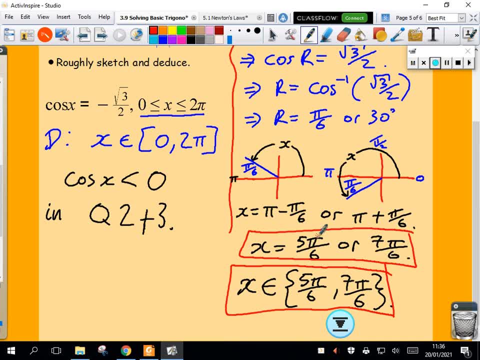 All the way down. And then when you have your final answer. In degrees. Well you just convert it. Into radians. At that stage. 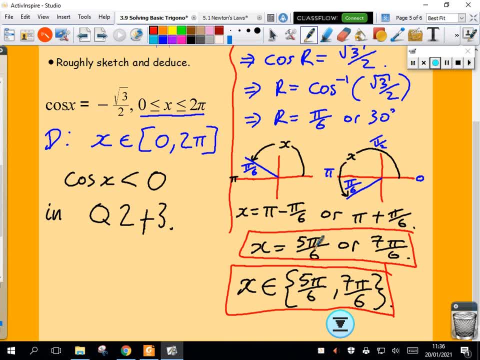 So you would find. This would be 150 degrees. This would be 210 degrees. Multiply by pi over 180. To convert into radians. Okay. So solving. Same few steps. All the time. 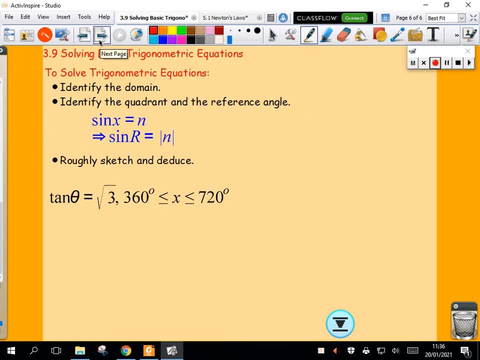 Let's look at one with the tan function. Again the same thing. Start by identifying the domain. I want to. I want to. Solve this equation. 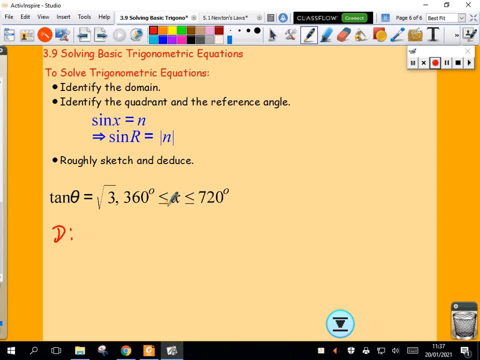 Tan of theta is root three. Notice theta has to be between 360 and 720. 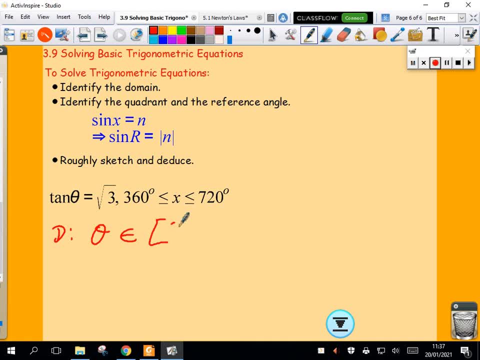 So. Theta. Belongs to the interval. Starting at 360. And finishing at 720. Why square brackets. Because 360 is included. Because it's a less than or equal to. That's step one. 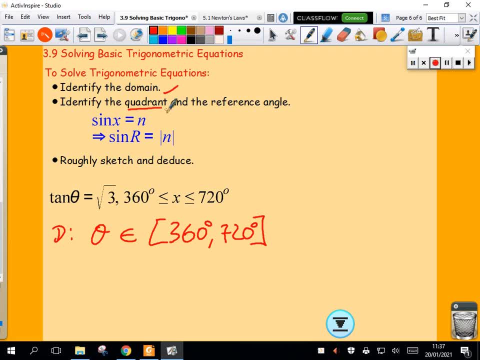 Identify the domain. Step two. Identify the quadrant. And then the reference angle. Okay. Well. To identify the quadrant. 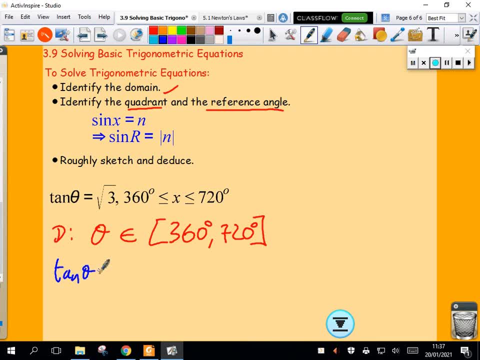 Tan is positive here. Tan of theta is positive root three. So we know that tan is positive in quadrants. And again. 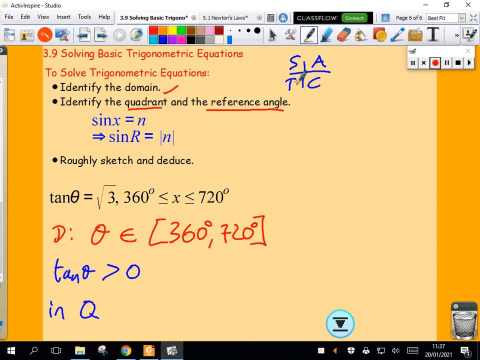 If you're unsure. You should know this stuff. If you're unsure. Have a quick look here. Tan is positive. 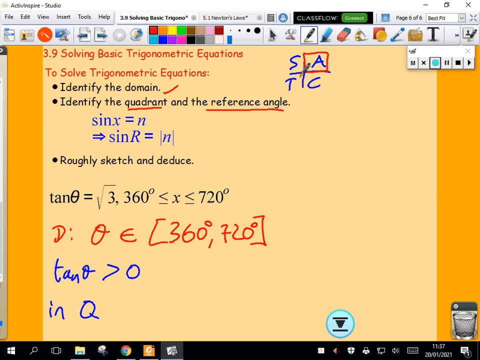 Well all functions have positive ratios in quadrant one. And only tan and its inverse. Or its reciprocal I should say. Have positive ratios in quadrant three. So we're dealing with quadrants one and three. 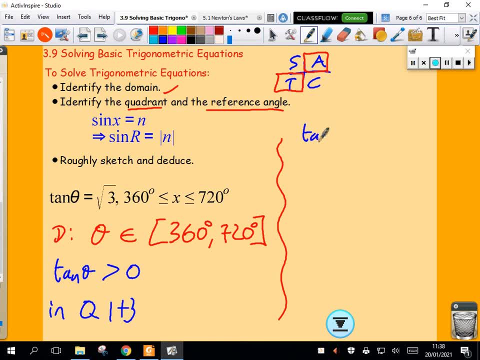 The reference angle. While tan of theta is equal to root three. Which means the tan of the reference angle. Is also equal to root three. 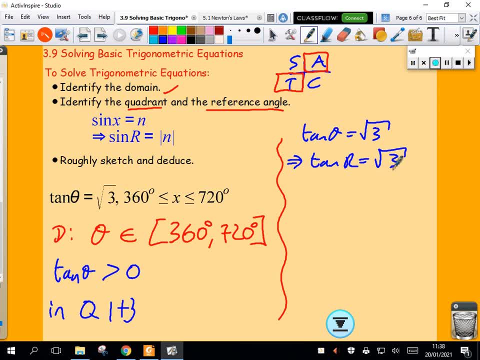 Remember the absolute value. Of a positive number. Is just that number itself. 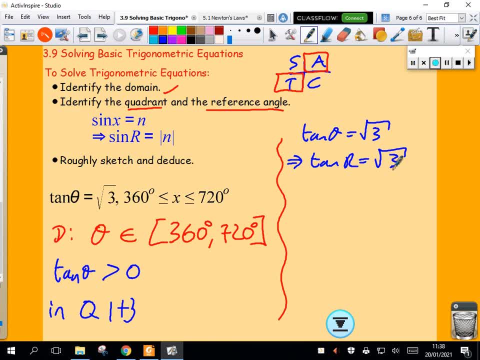 The absolute value of a negative number. Is the opposite of that number. 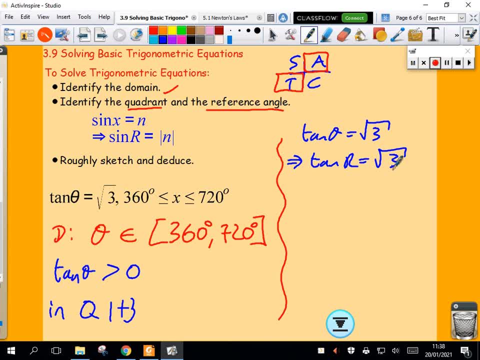 I'm also in degrees here. So one thing I'm going to make sure. If I'm using a calculator. 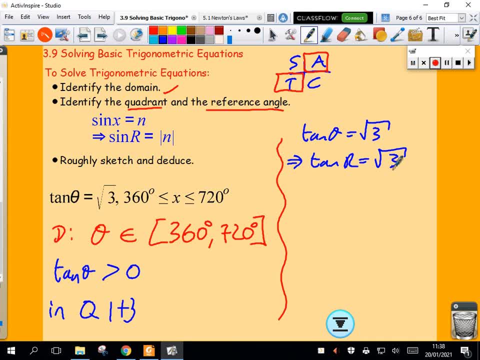 Which I shouldn't really need to use. If I know my special angles well enough. 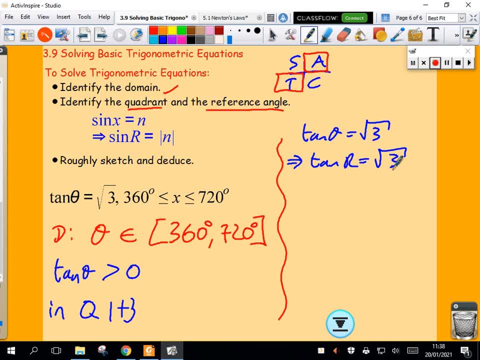 But I'm using a calculator. If I'm using a calculator. 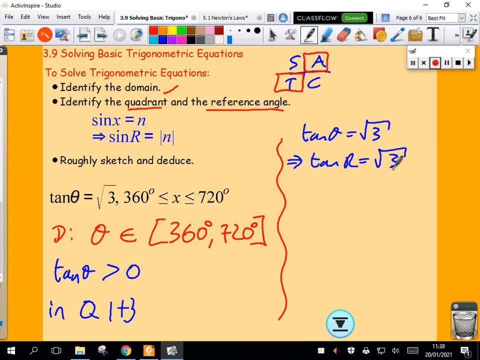 I want to make sure it's in degree mode. Okay. So in my calculator. I put it in degree mode. It's shift setup. 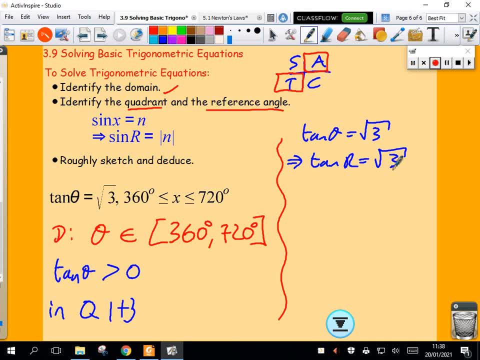 And then number two for the angular Newton. And number one for degrees. 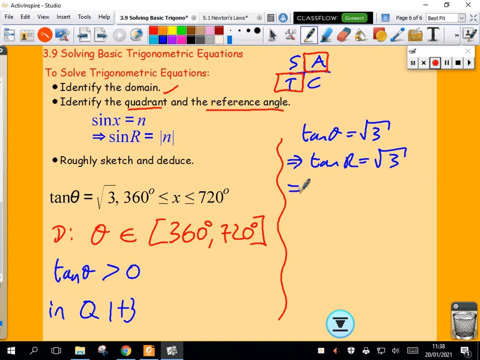 Okay. So you should know this. If you don't. 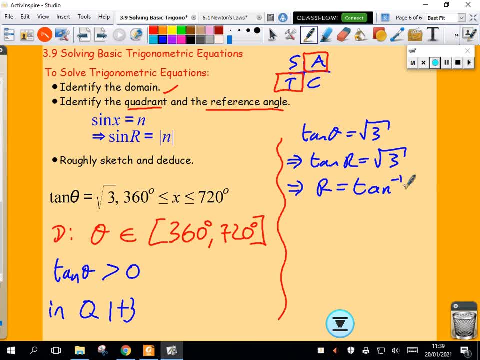 You just type into your calculator. The reference angle is going to be. Tan inverse of root three. Okay. 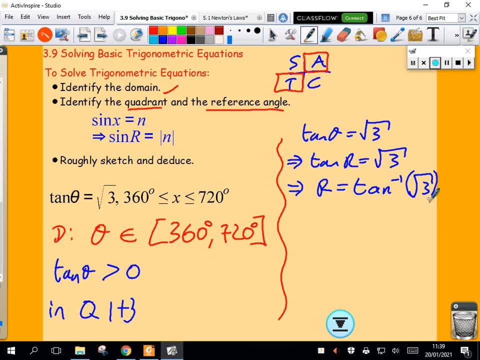 So tan inverse of root three. Into your calculator. 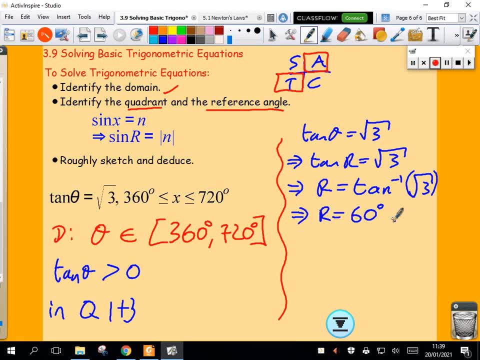 You'll find that the reference angle. Is sixty degrees. Okay. 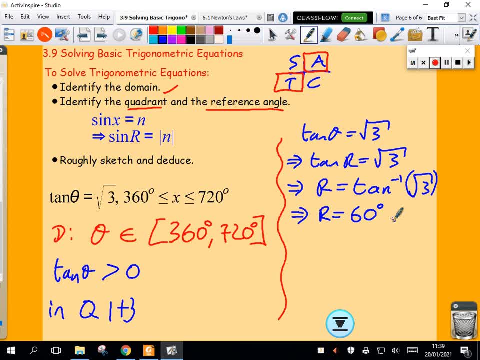 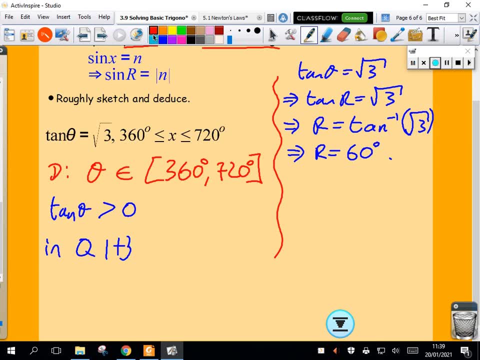 So we've identified the quadrant. We've identified the reference angle. We've identified the domain. Now we want to go and sketch. Okay. 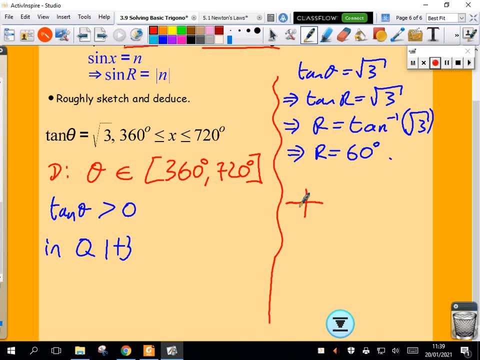 So two quadrants here. Two quadrants here. Just a rough sketch will do. 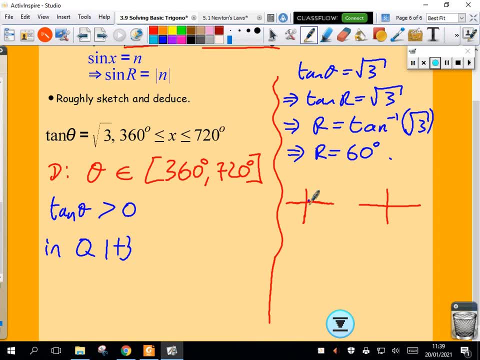 Either quadrant one. With a reference angle of sixty degrees. Well there is quadrant one. With a reference angle of sixty degrees. Or quadrant three. 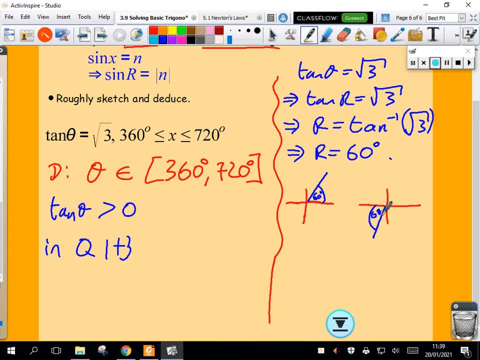 With a reference angle of sixty degrees. reference angle of 60 degrees in there. 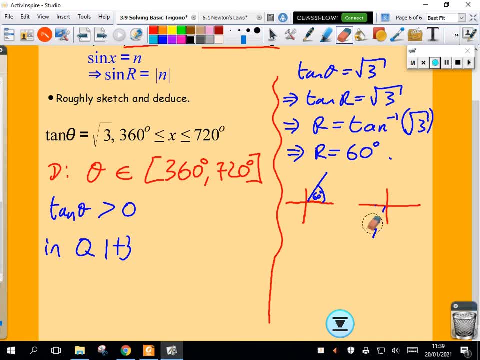 Write that in again. It's a little... It doesn't look great. 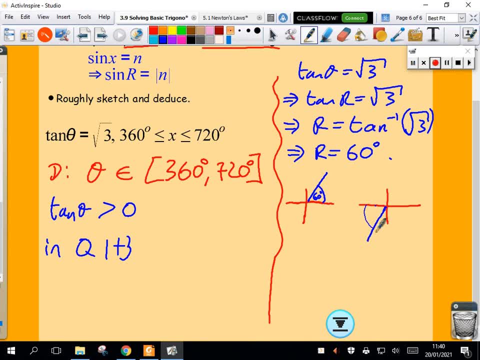 I'm going to make my pen a little narrower, so 60 degrees in there. 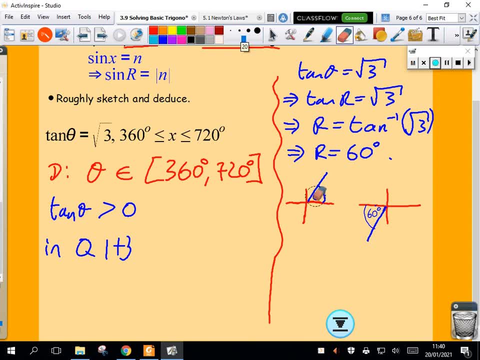 Okay. And I'll do the same with this one. It's just a little difficult to see at the moment. So 60 degrees in there. Okay.